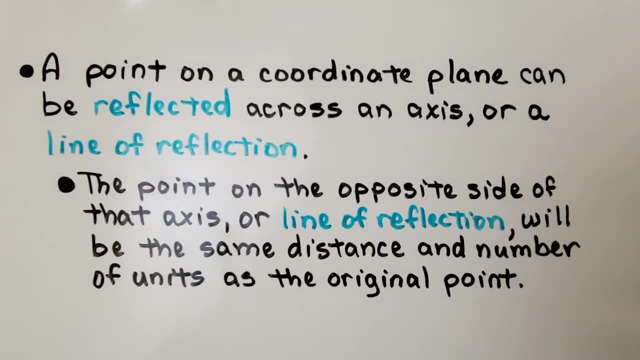 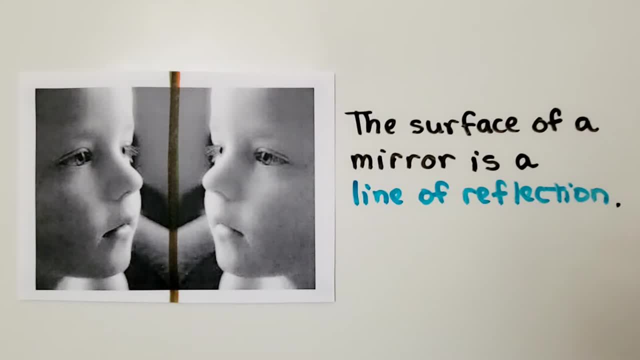 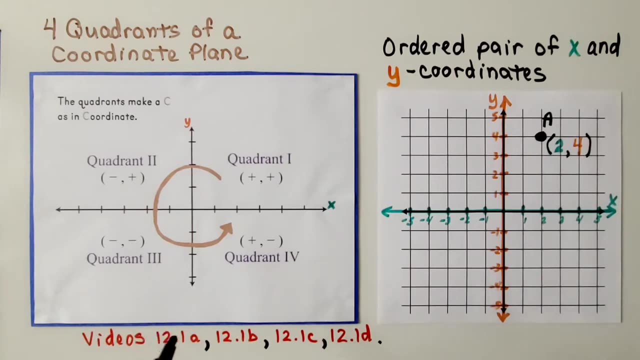 be the same distance and number of units as the original point. When you look in a mirror, you're looking at your reflection and the surface of a mirror is a line of reflection. Back in 12.1,- all the parts of 12.1,, we learned about the four quadrants of a coordinate plane. 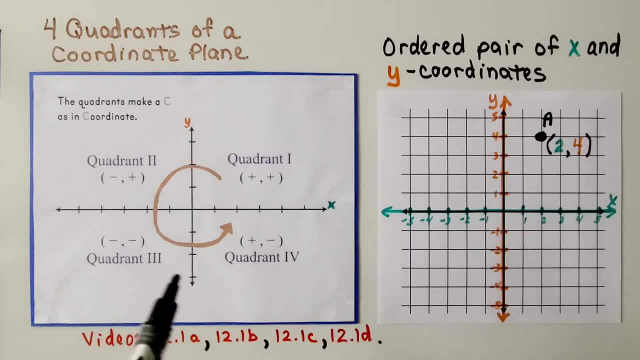 This is quadrant 1, and it goes around to 2,, 3, and 4.. They're written in Roman numerals And it makes the shape of a C, like in the word coordinate, so you can easily remember, And an ordered pair of. 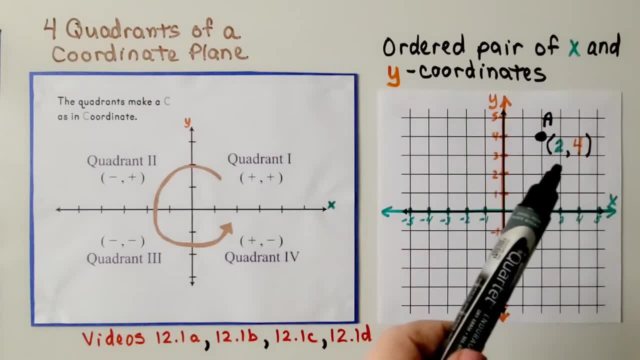 X and Y coordinates with the X first, and then the Y will show us where a point is. This point A is at 2 for X, so here's the X axis, We go to a positive 2, and it's at 4 for Y, so we go up to 4 on the Y and there's our point A. So here we have point A and 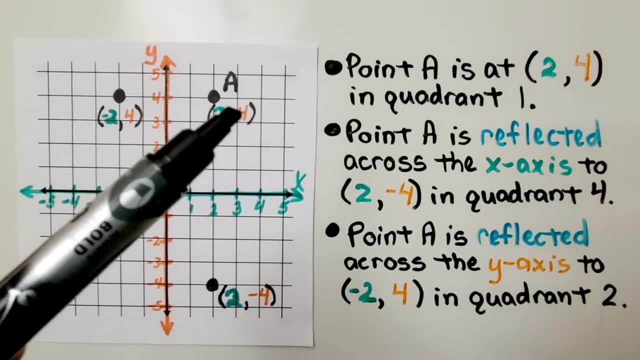 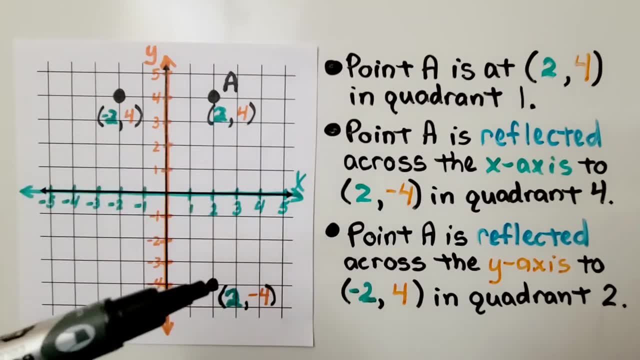 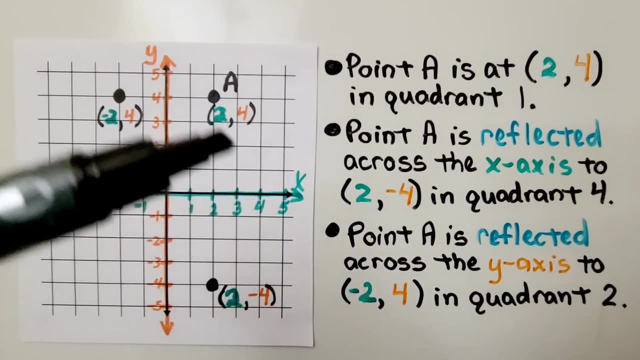 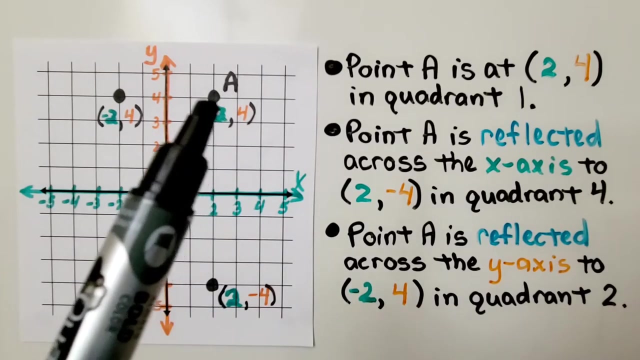 it's located in the first quadrant at 2 for X and 4 for Y, And point A is reflected across X axis to 2 for X negative 4 for Y. So this point is a reflection across the X axis of point A. We can see that this is in quadrant 4.. If we reflect point A across the Y axis, 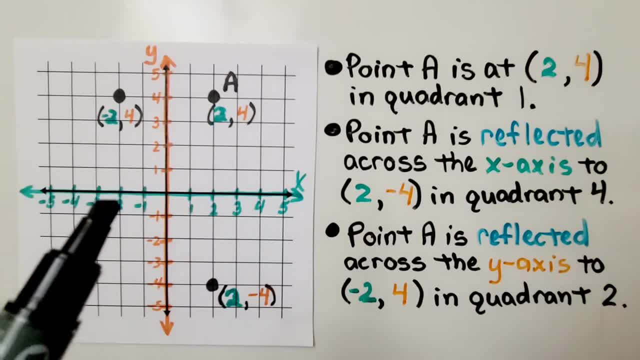 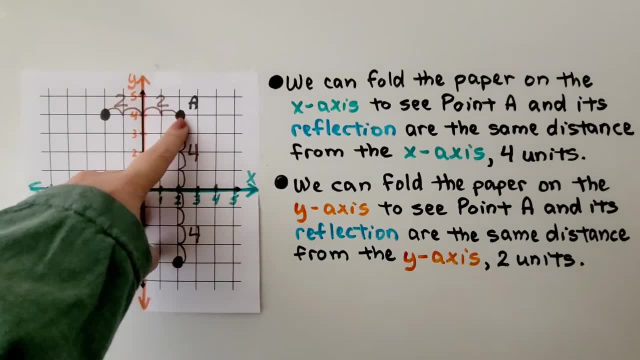 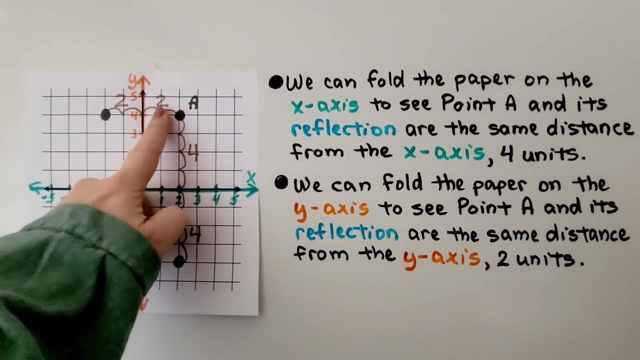 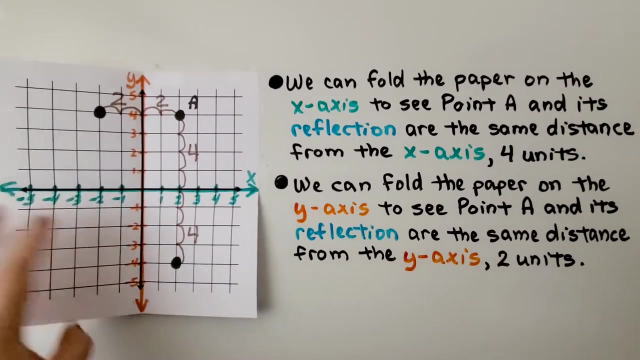 it's over here in quadrant 2 at negative, 2 for X and 4 for Y. Here we have point A and its reflection across the x-axis to here, and then another reflection of a across the y-axis to here, and we can fold the paper on the x-axis to see point a and its reflection. 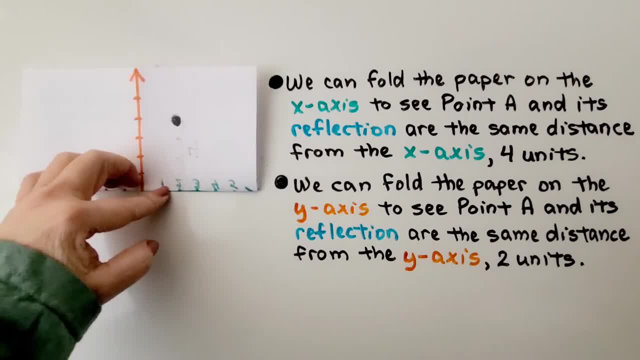 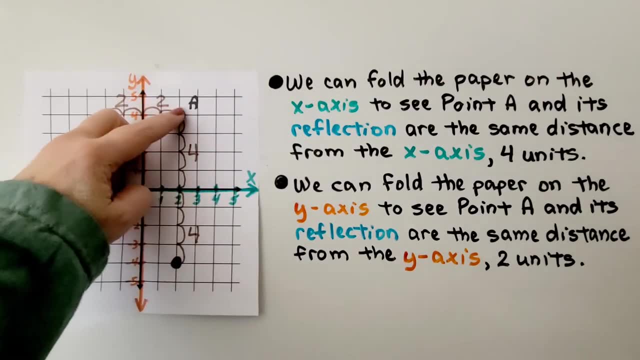 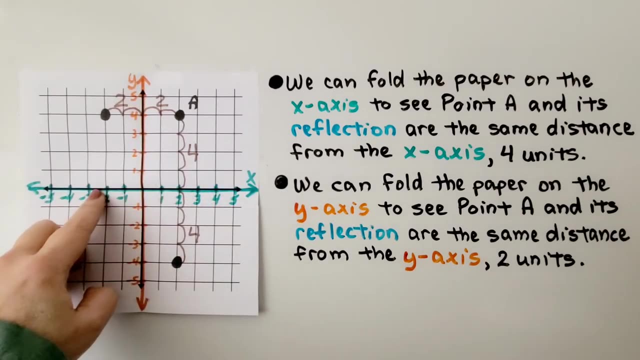 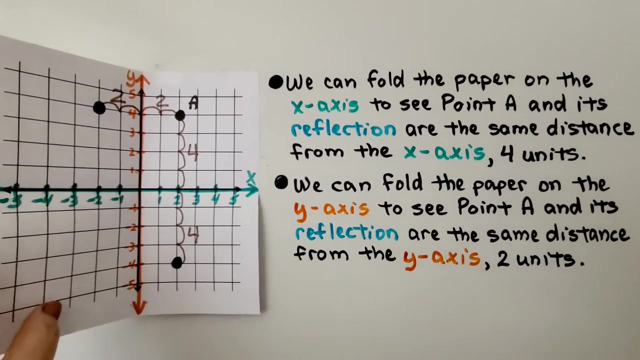 are the same distance from the x-axis. it's one, two, three, four. and it's one, two, three, four, it's four units from this line of reflection, the x-axis. we can also fold the paper on the y-axis this way as the line of reflection, and we can see point a and. 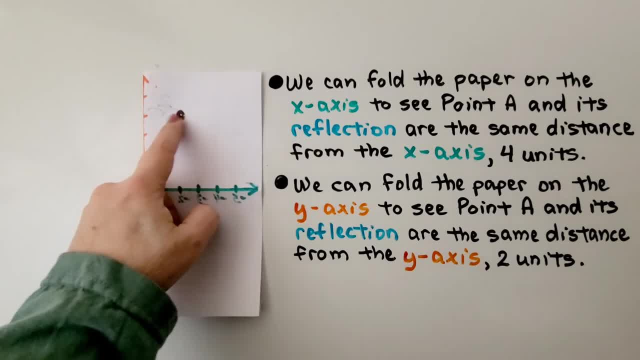 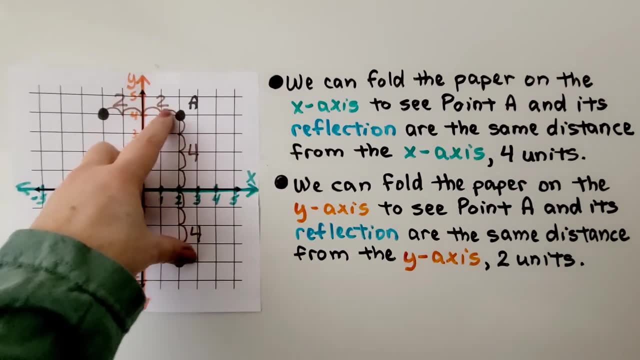 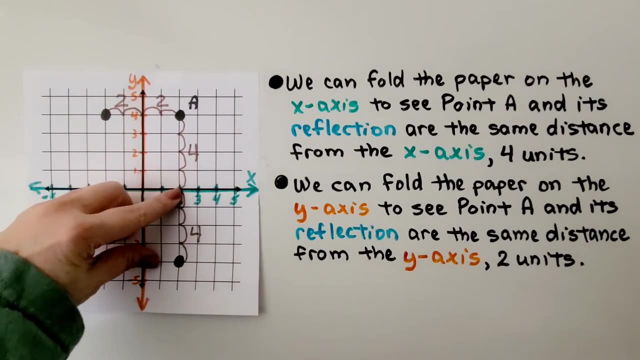 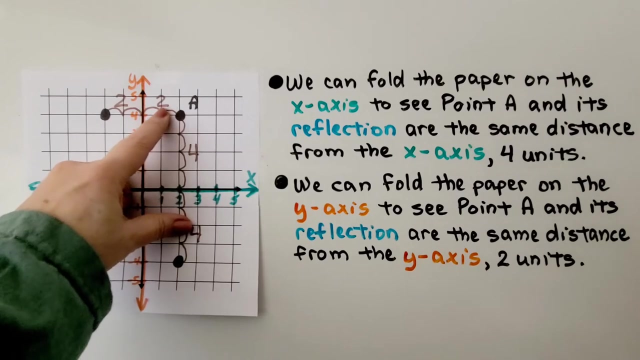 its reflection are in the same distance from the y-axis: two units. it's one, two, one, two, one, two, and we don't need to fold the paper. we can look and see that this is four units from x and this one is four units from x. we can see this one is two units from y and the reflection is two units. 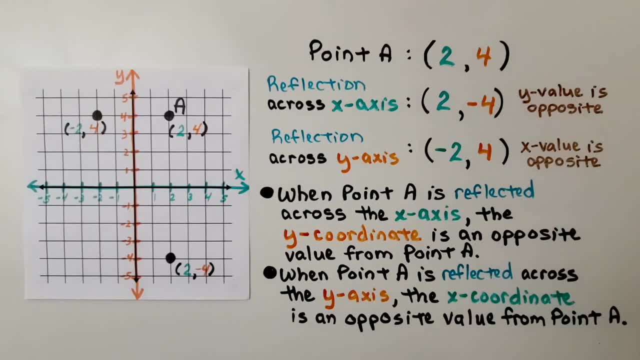 from y. the x and y coordinates for point a are two for x, four for y, two for x and four for y. the reflection across the x-axis is two for x and negative four for y. the y value is opposite of point a. this is a positive four. 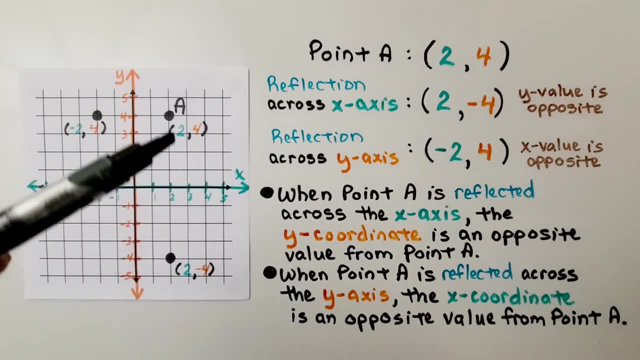 now it's a negative four, but they both have a positive two for an x value, the reflection across the y-axis. now we have a negative two and a positive four. so now this negative two is opposite of this positive two and they both have a positive four. 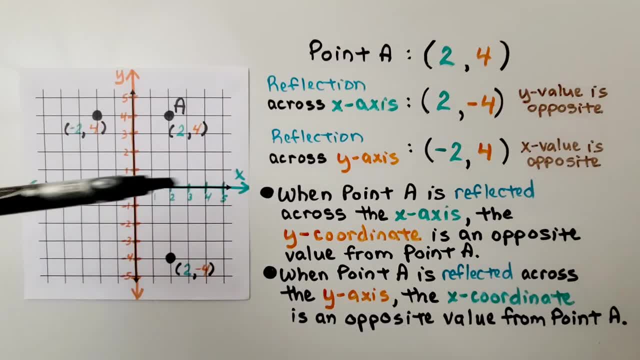 when point a is reflected across the x-axis, the y-coordinate is an opposite value from the y-coordinate in point a, and when point a is reflected across the y-axis, the x-coordinate is an opposite value from point a. we have a positive two. now it's a negative two. 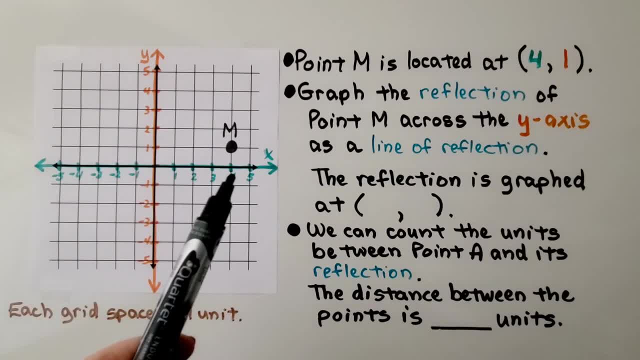 here we have point m and it's located at four for x and one for y. we need to graph the reflection of point m across the y-axis as a line of reflection. we know it's going to be the same distance from y as point m. this is one, two, three, four units away. 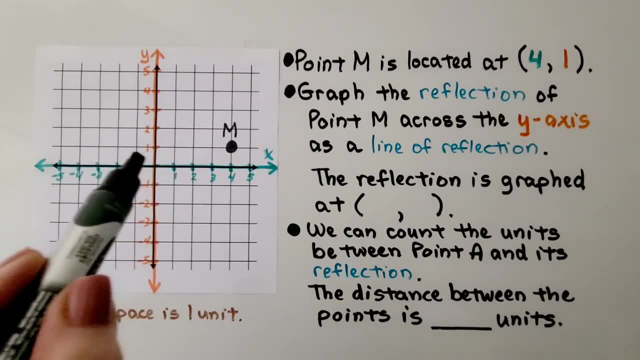 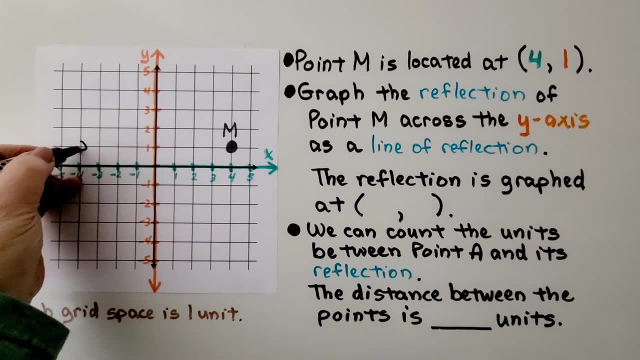 from y and it's going to still be on one. it's going to come straight across like that: we need to count one, two, three, four units. on the opposite side, that would be the reflection of point m, and the reflection is graphed at negative four for x.